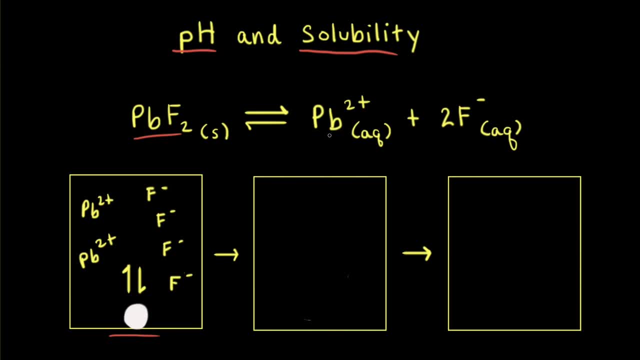 with the ions in solution Lead, two fluoride forms lead, two plus ions and fluoride anions in a one to two mole ratio. So if we have two lead two plus ions in this diagram, we need four fluoride anions At equilibrium. the rate of dissolution. 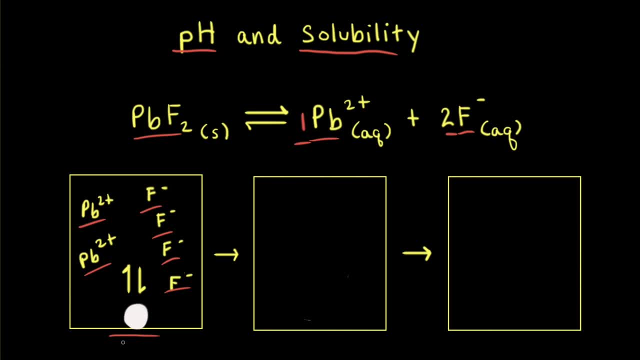 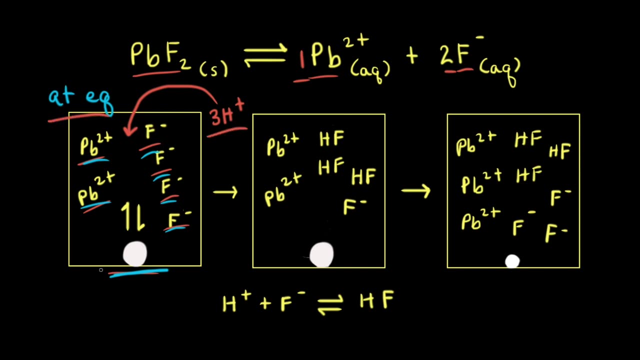 is equal to the rate of precipitation and therefore the amount of solid and the concentration of ions in solution remains constant, And this forms a saturated solution of lead, two fluoride To the system at equilibrium. we're gonna add some H plus ions, So by increasing the concentration, 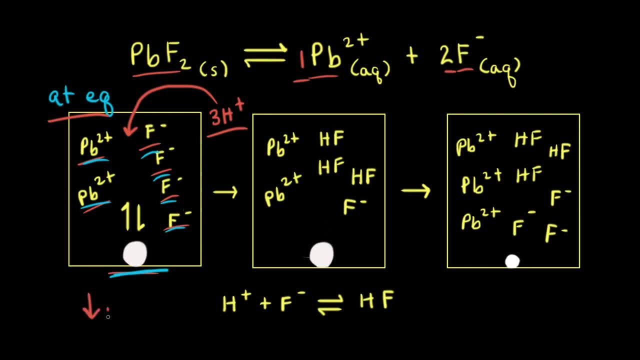 of H plus ions in solution, we're decreasing the pH of the solution. When the H plus ions are added to the solution, most of them react with the fluoride anions that are present. So H plus plus F minus forms HF. Comparing the first diagram to the second diagram: 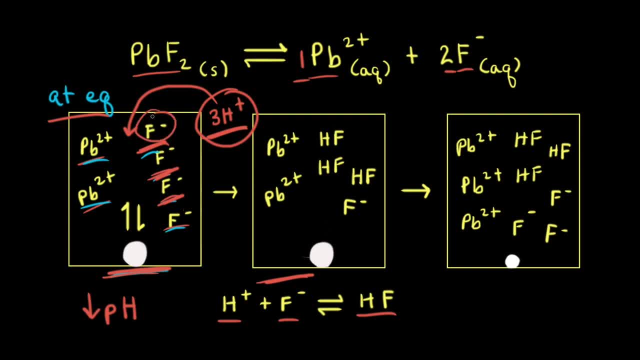 I just happened to add three H plus ions, which will react with three of the fluoride anions that are present to produce three HF. Notice how the concentration of fluoride anions in solution has decreased from the first diagram to the second diagram because of the addition of the H plus ions. 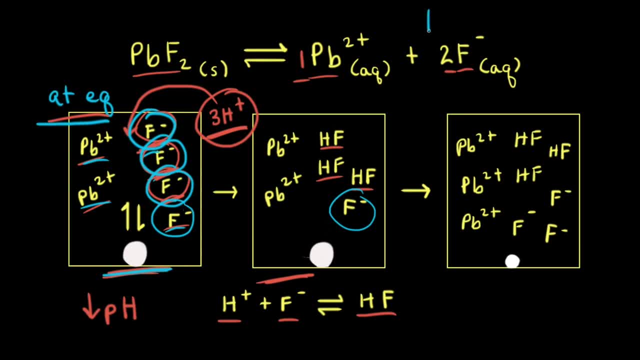 So the system wasn't. it was at equilibrium and the concentration of fluoride anions was decreased. According to Le Chatelier's principle, the system will shift in the direction that decreases the stress. So, if the stress is decreased, concentration of fluoride anions. 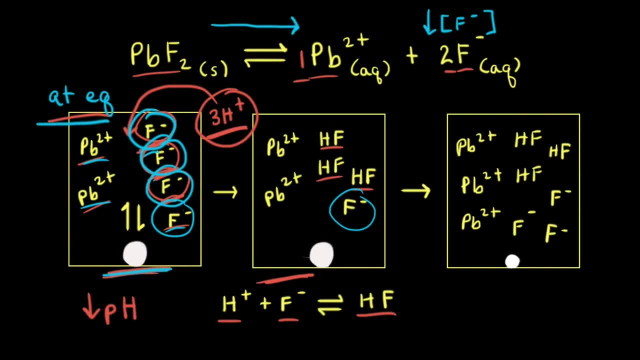 the system will shift to the right to make more fluoride anions And when the system shifts to the right, more lead to fluoride dissolves to increase the concentration of PB2 plus and fluoride anion. We can see that comparing the second diagram to the third diagram. 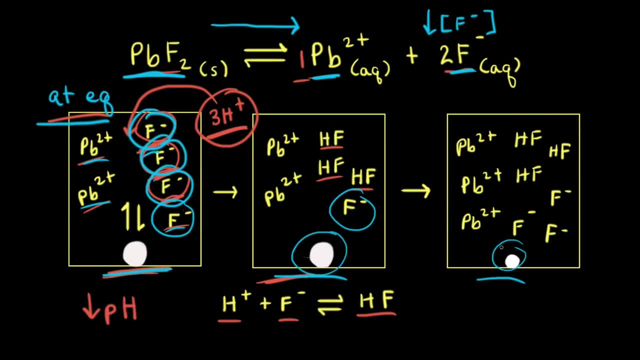 So the amount of solid has gotten smaller. since some of that lead to fluoride dissolved and we've increased the concentration of PB2 plus and F minus in solution, The solid keeps dissolving and the concentration of ions keeps increasing in solution until the system reaches equilibrium. 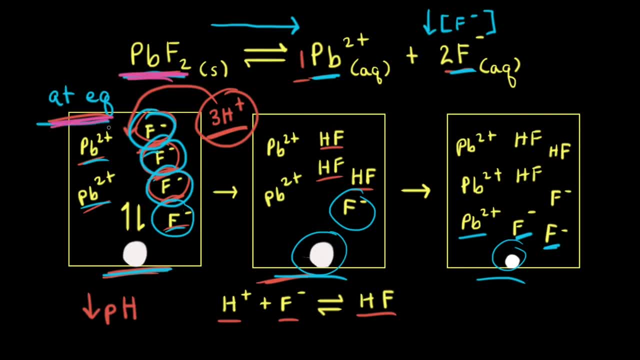 So for a saturated solution of lead to fluoride at equilibrium. decreasing the pH or making the solution more acidic by increasing the concentration of H plus ions increases the solubility of lead to fluoride, which is why we saw more of the solid dissolve. 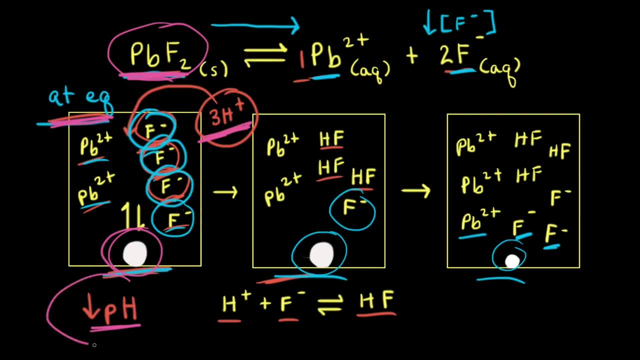 when the H plus ions were added. This effect of decreasing the pH and increasing the solubility of a slightly soluble salt happens whenever the slightly soluble salt contains a basic anion. For this example, the basic anion is the fluoride anion. 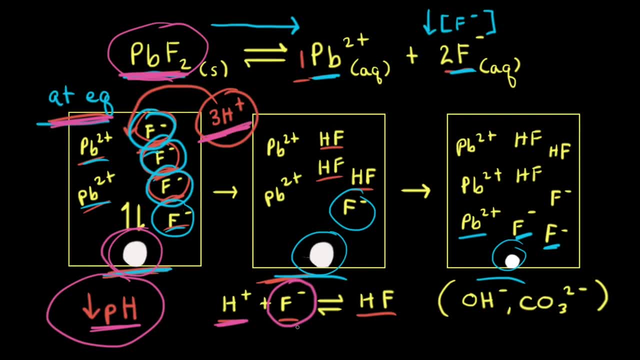 which reacts with the added H plus ions, And when the basic anion reacts, that decreases the concentration of that basic anion which caused the equilibrium to shift to the right. And there are many other examples of basic anions. Two more would be the hydroxide anion. 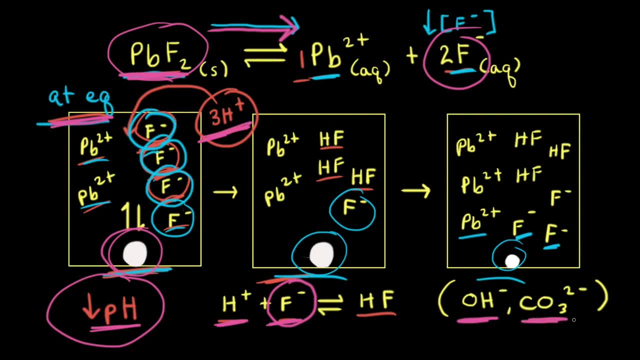 and the carbonate anion, And if a compound contains a basic anion such as the hydroxide anion, hydroxide functions as a base and reacts with H plus ions to form H2O. So therefore, the solubility of a compound containing 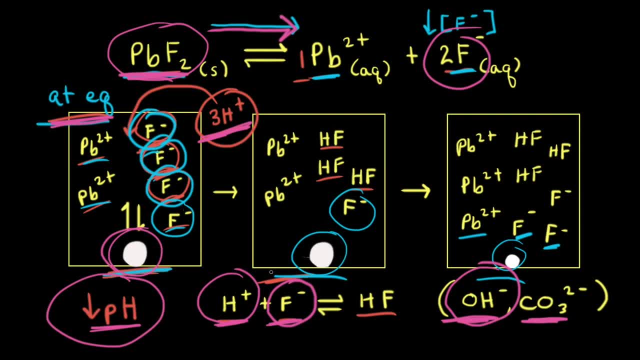 a hydroxide ion would increase as H plus ions are added to the solution. It's also important to note, for this lead to fluoride problem. if the pH is decreased at a constant temperature, the KSP value for PBF2 remains constant. 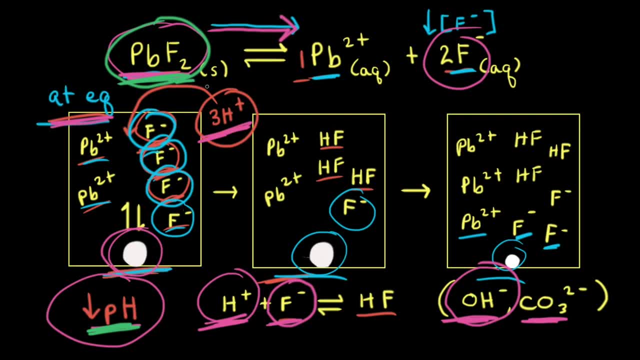 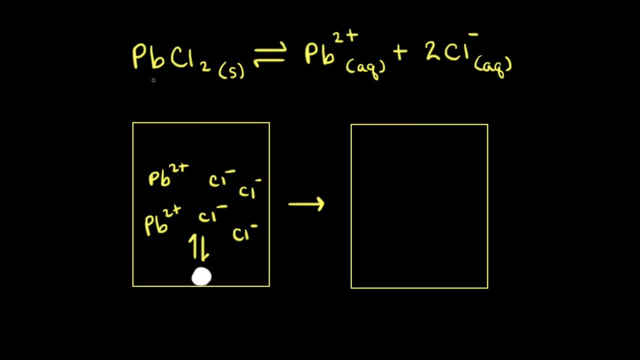 So the molar solubility does increase, but the KSP value remains the same. This time, instead of lead to fluoride, let's look at lead to chloride. Lead to chloride is also a white solid, So if we dissolved some in solution, 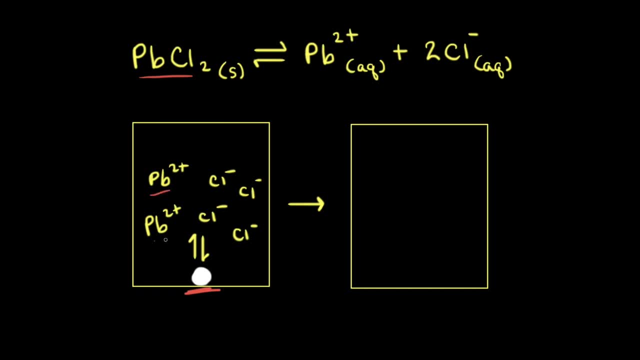 eventually we would reach an equilibrium between the solid and the ions in solution. So this diagram here shows a saturated solution of lead to chloride and the system is at equilibrium, And to the system at equilibrium. we decrease the pH by adding H plus ions to the solution. 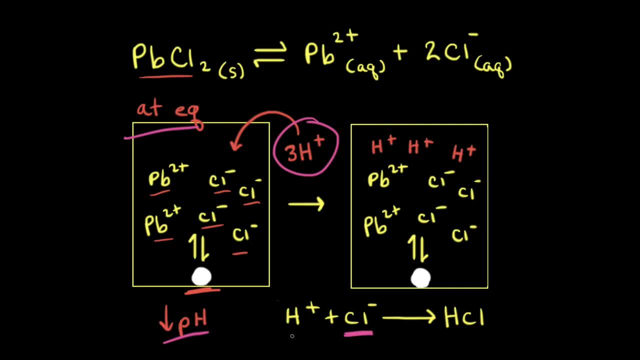 In this case, the chloride anions aren't basic enough to react with the H plus ions. Therefore, we do not form HCl And the concentration of chloride anions remains the same as it was in the original diagram. So if the concentration of chloride ions remains the same, 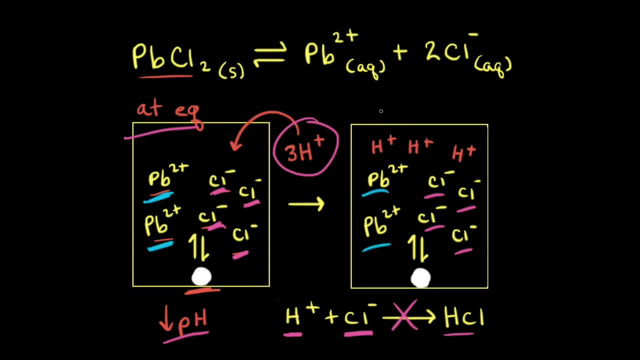 and the concentration of lead to plus ions would remain the same. the system is still at equilibrium, and decreasing the pH had no effect on the solubility of the solids. So we have the same amount of lead to chloride solid on the bottom of the beaker in both diagrams.